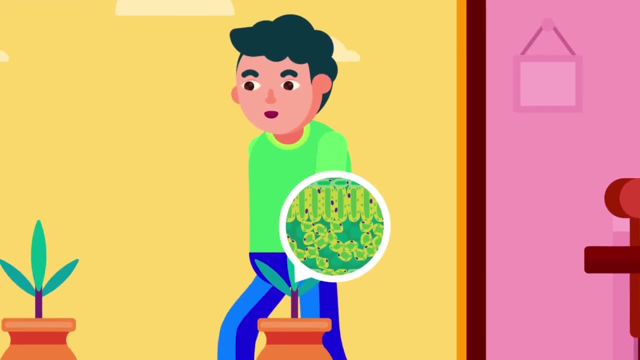 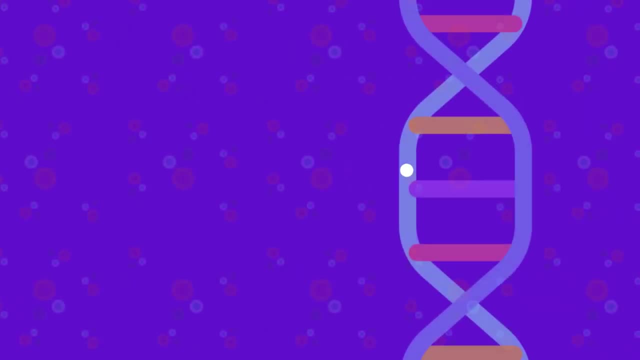 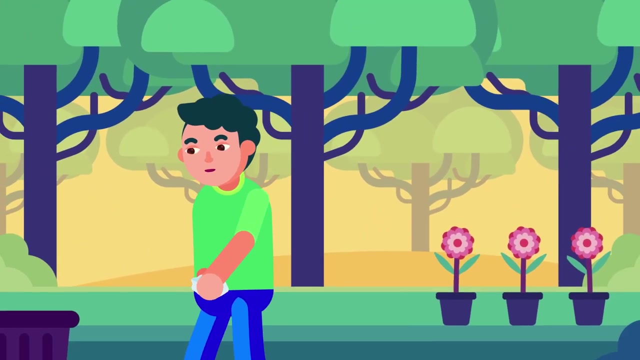 as supporting structures like, for example, cellulose cell walls in plants. They are used to make other organic compounds like amino acids and fats. Nucleic acids like DNA are also formed by carbohydrates, as well as lubricants like mucus, Another fascinating function of 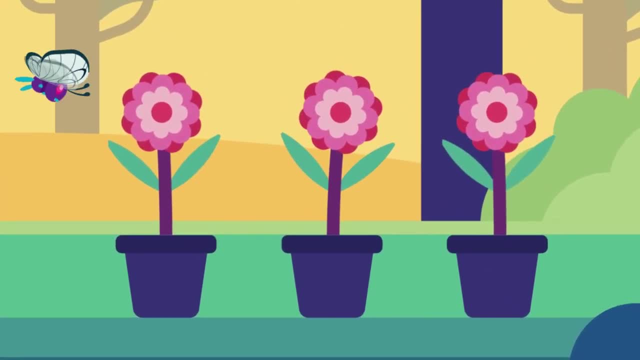 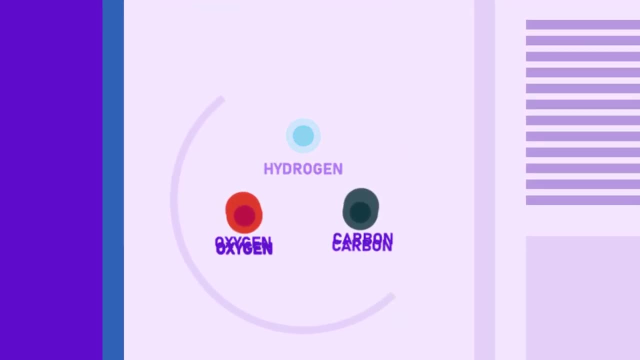 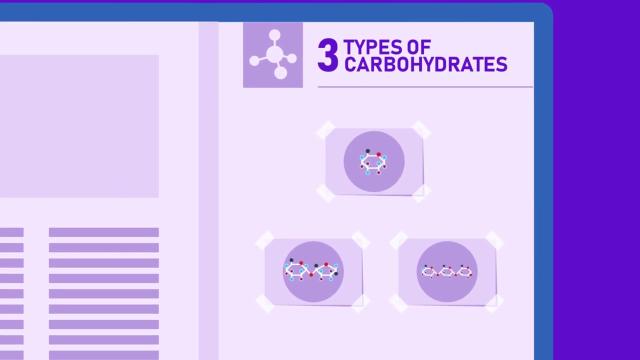 carbohydrates is that they are also used to produce the nectar in some flowers. Carbohydrates are organic compounds made up of carbon, hydrogen and oxygen. The hydrogen and oxygen atoms are present in the same ratio, that is, 2 to 1.. There are 3 main types of carbohydrates. 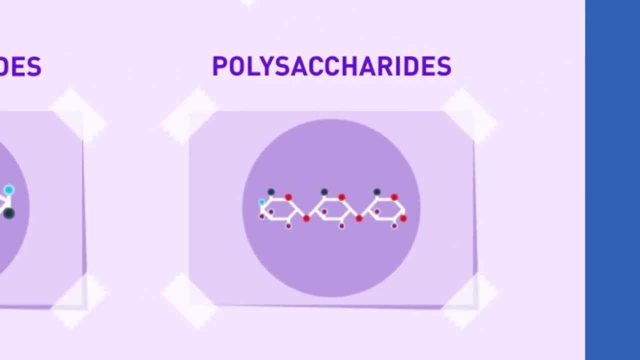 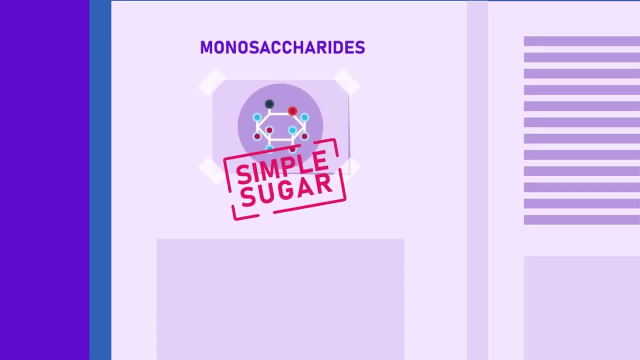 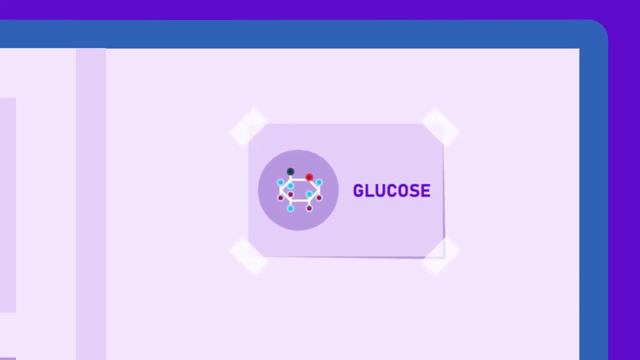 – monosaccharides, disaccharides and polysaccharides. Monosaccharides have a simple chemical composition and therefore known as simple sugars. Examples of them are glucose, fructose and galactose. The sugar glucose is one of the simplest forms of sugars and has the chemical formula C6H12O6. 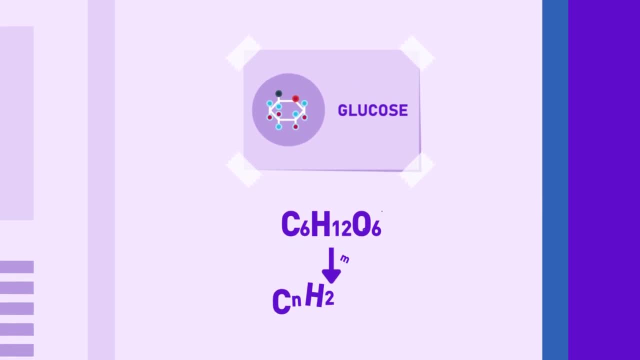 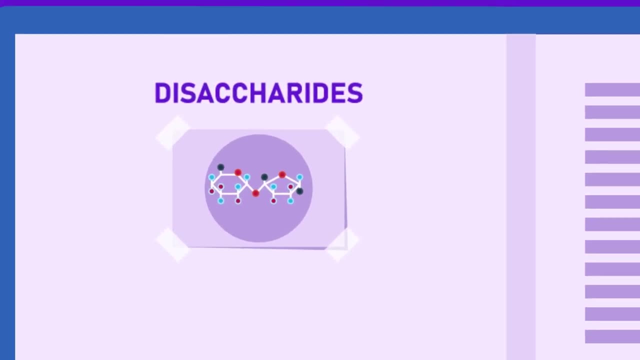 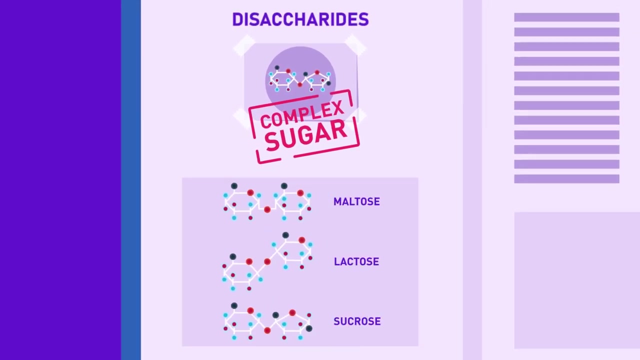 The generalized formula for carbohydrates is CNH2MOM. In the case of glucose N and M is equal to C6H12O6.. Disaccharides are also known as complex sugars, as they have complex chemical compositions. Maltose, lactose and sucrose are their examples. Disaccharide structure molecules are made. 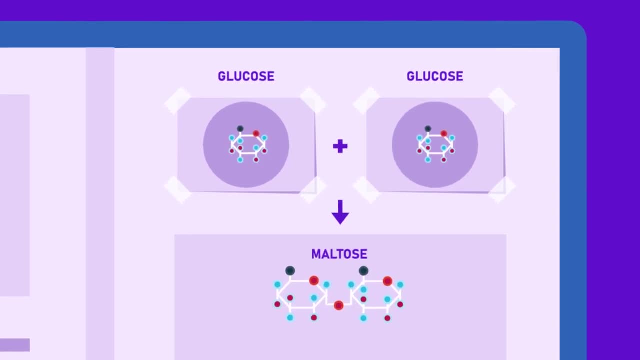 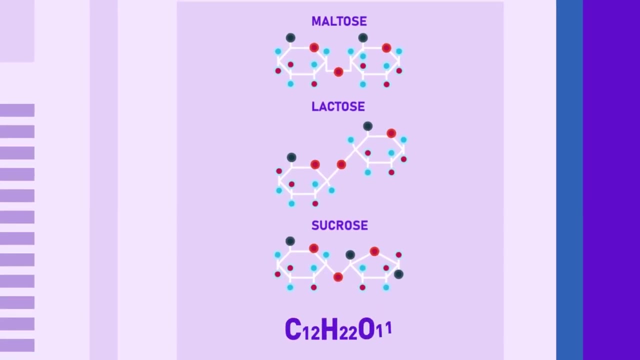 up of two molecules of simple sugars condensed together. The most common types of disaccharides have 12 carbon atoms with the general formula C12H22O11.. The differences in the disaccharides are again due to the different atomic arrangements within the molecule. 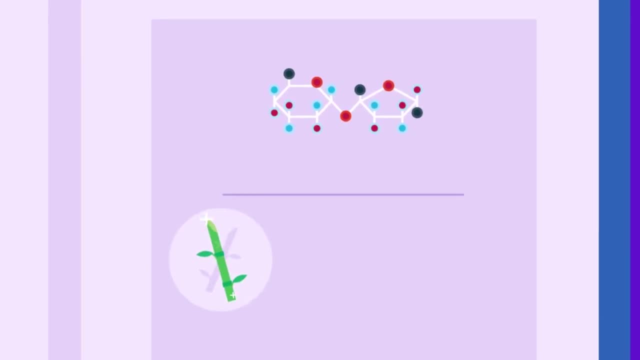 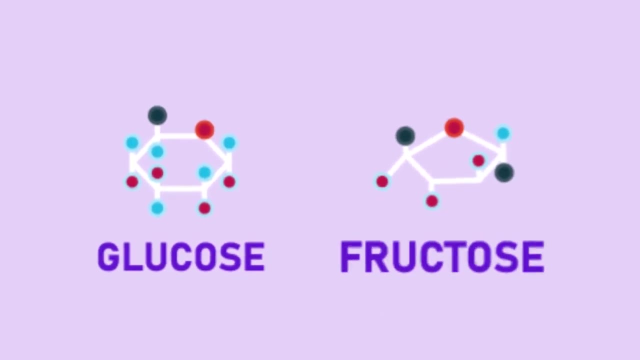 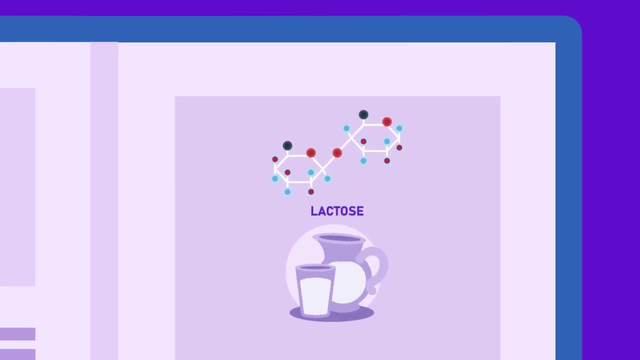 Glucose, or cane sugar, occurs in sugar cane stems, sweet fruits and certain storage roots, for example carrots. It consists of a glucose and a fructose molecule combined together. Lactose, also known as milk sugar, is commonly found in milk. as the name suggests It is. 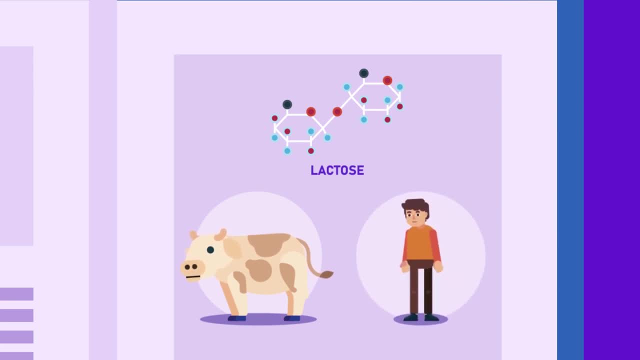 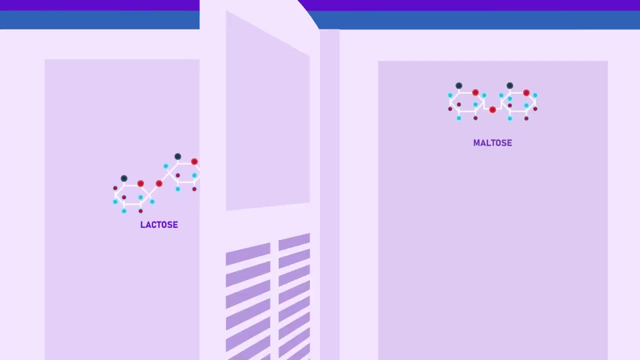 found in milk of all mammals, including humans, and even in some similar fluids, such as pigeon's milk. It is formed from glucose and galactose combined together. Maltose, known as malt sugar, is present in malted cereals and sprouting grains. It